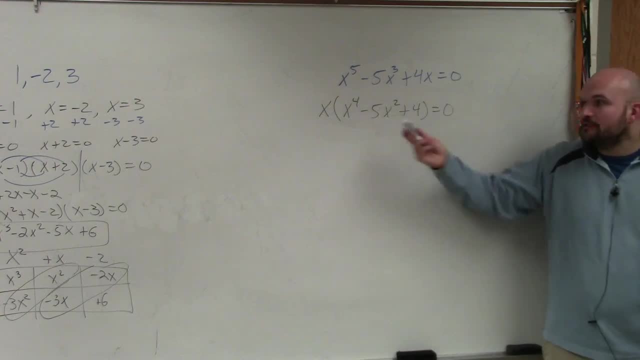 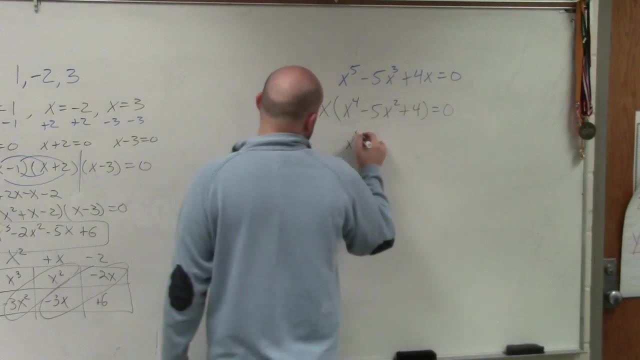 Right. So again, ladies and gentlemen, you have a product equal to 0.. So you can set those both equal to 0 by using the zero product property. So you have x equals 0 and x to the 4th minus 5x. squared plus 4 equals 0.. 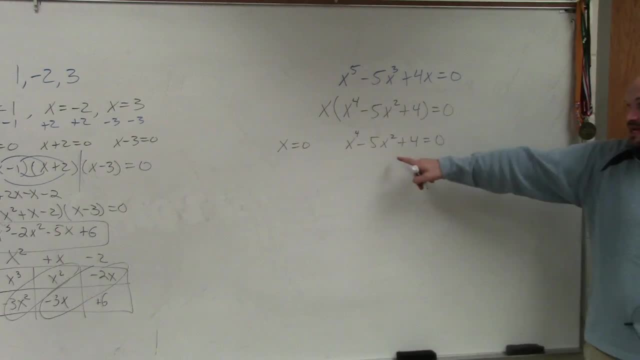 Well, ladies and gentlemen, this is still something that needs to factor. We can't solve for x like this. So what I told you, What I told you guys to do is, when you have a polynomial to a higher power, notice, I can't factor anything else out. 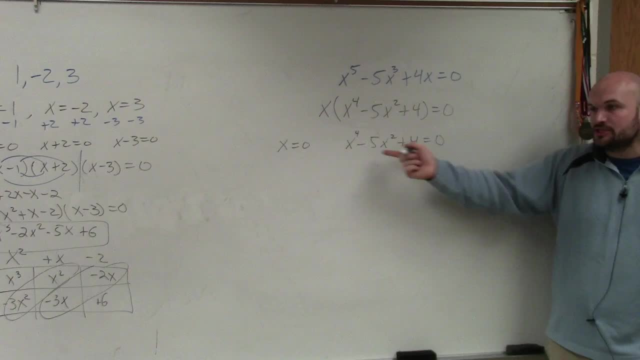 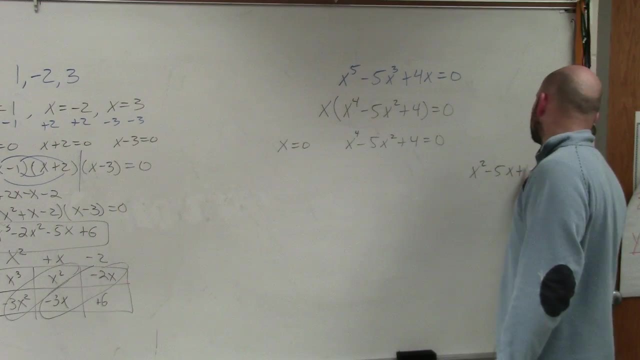 So what I said was: look at, think of it as like a quadratic. If it's a trinomial, think of it like a quadratic. So if I wanted to just factor x squared minus 5x plus 4, if I was just going to factor that, I could factor, did anybody? 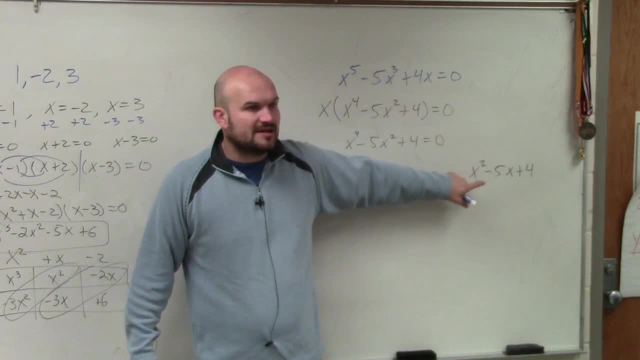 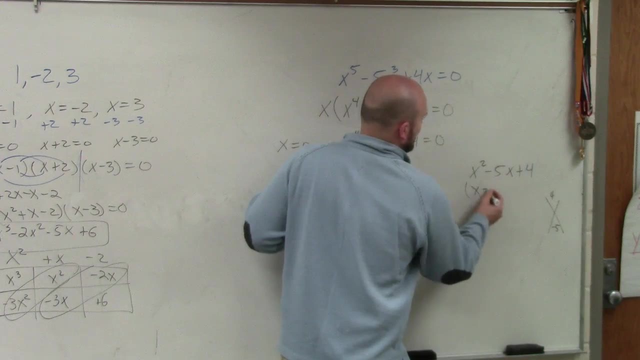 a lot of people got this one factored. The factored form of this would be: what two numbers multiply to give you 4, add to give you 0. And the answer is negative 4.. The answer is x minus 4 times x minus 1.. 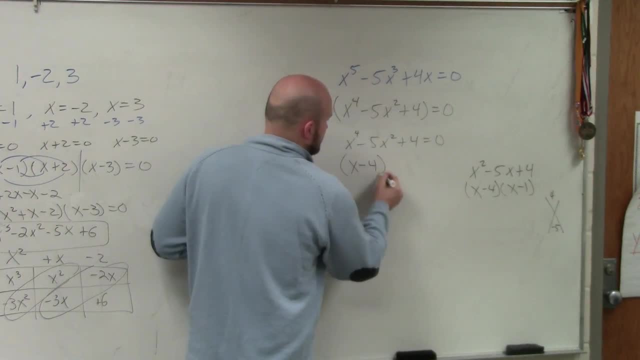 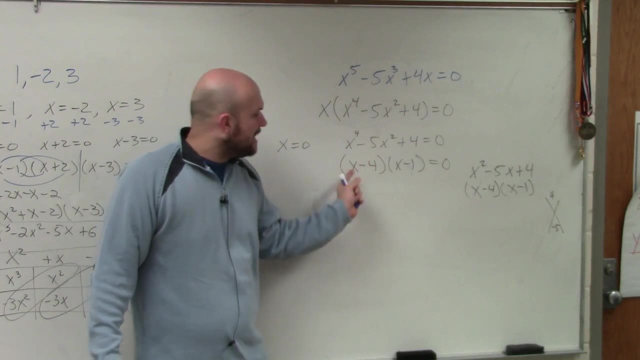 Right, So we could factor that like that. However, ladies and gentlemen, does x times x give you x to the 4th? No, So what power should I raise these to Squared And guess what That works now? 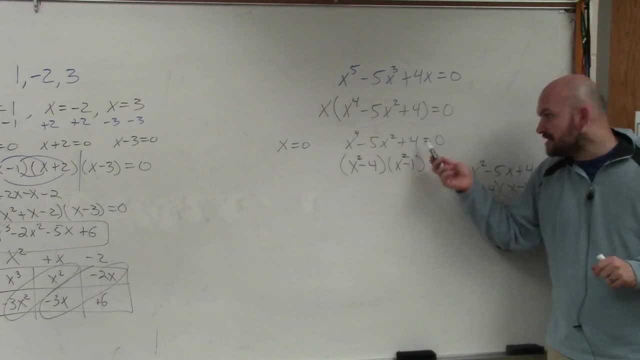 X squared. times x squared gives you x to the 4th. Negative 4 times negative: 1 gives you positive 4.. Negative 4 times x squared gives you x to the 4th. Negative 4 times x squared gives you x to the 4th. 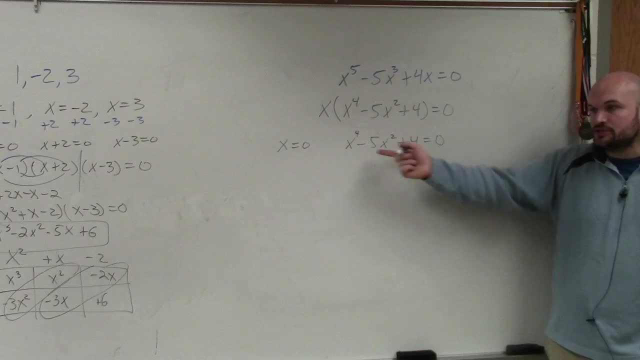 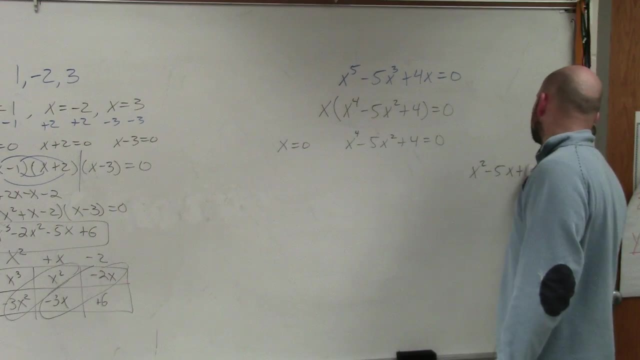 So what I said was: look at, think of it as like a quadratic. If it's a trinomial, think of it like a quadratic. So if I wanted to just factor x squared minus 5x plus 4, if I was just going to factor that, I could factor, did anybody? 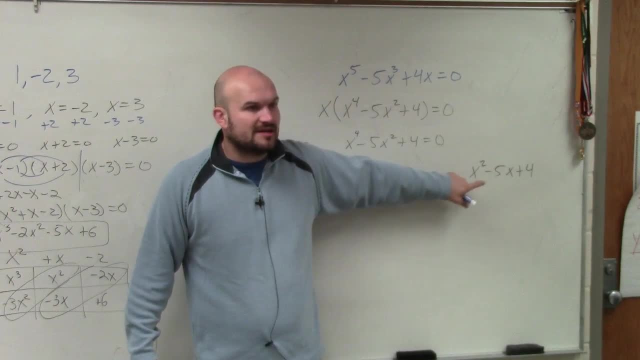 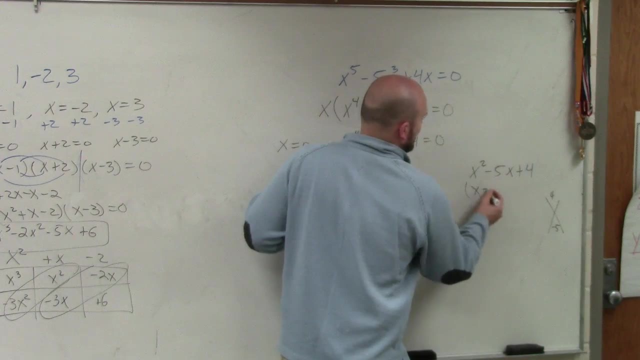 a lot of people got this one factored. The factored form of this would be: what two numbers multiply to give you 4, add to give you 0.. What's the answer? What's the answer? The answer is x minus 4 times x minus 1.. 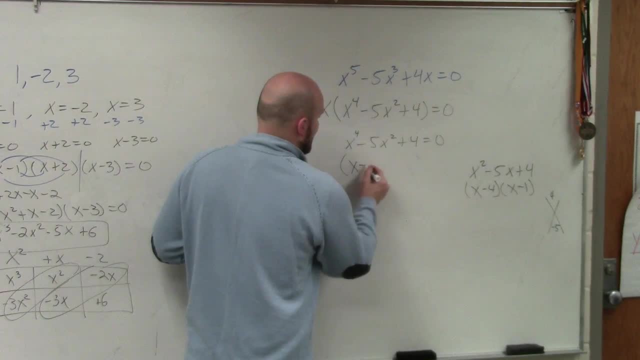 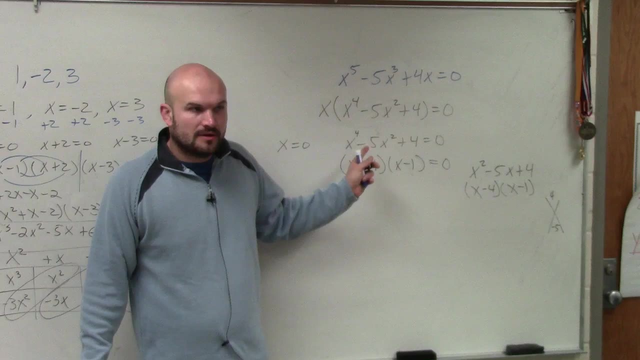 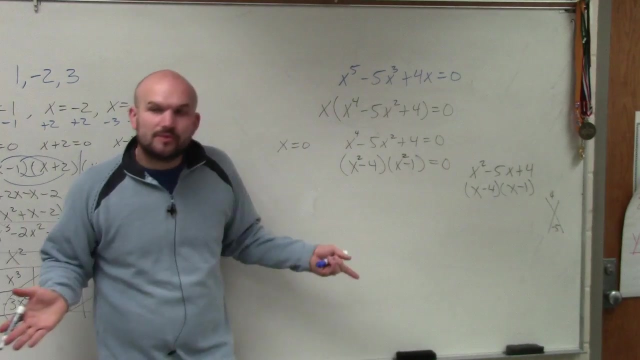 So we can factor that like that. However, ladies and gentlemen, does x times x give you x to the 4th? No, So what powers? should I raise these to Squared And guess what That works now? X squared times x squared gives you x to the 4th. 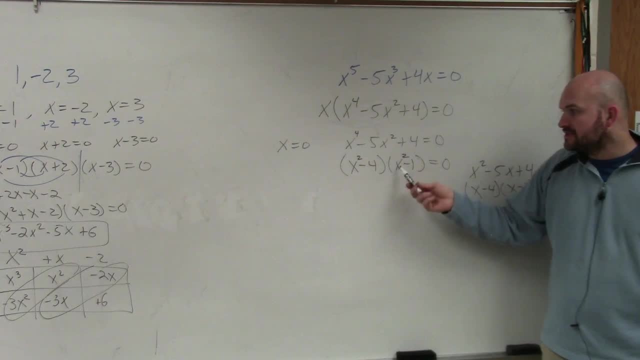 Negative 4 times negative 1 gives you positive 4.. Negative 4 times x squared gives you x to the 4th. Negative 4 times x squared, plus negative 1 times x squared, gives you negative 5x squared. Now I can apply the zero product property again. 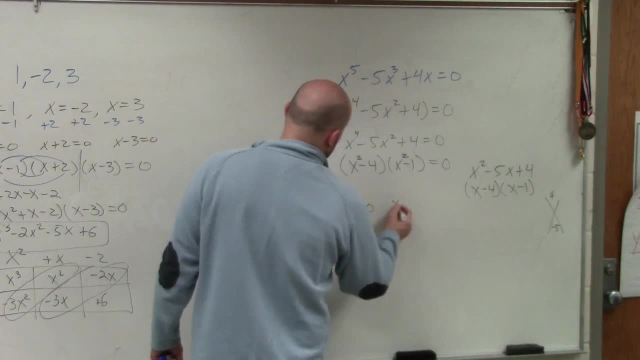 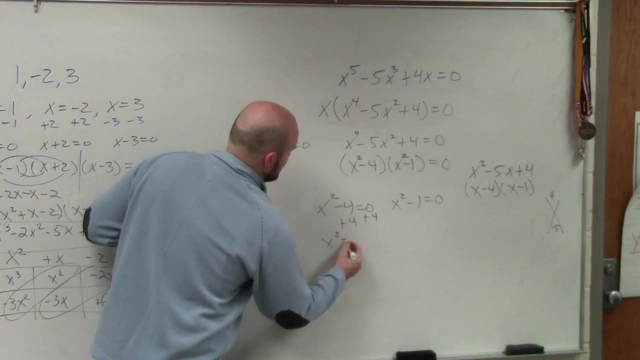 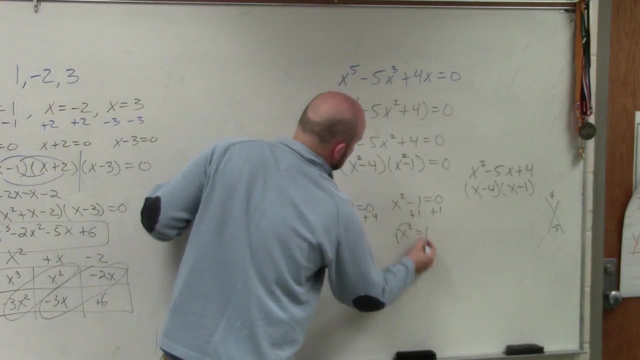 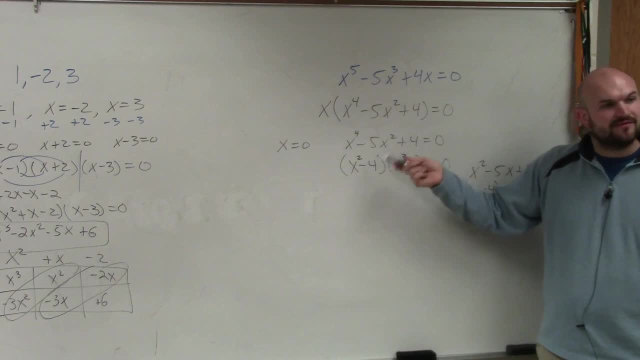 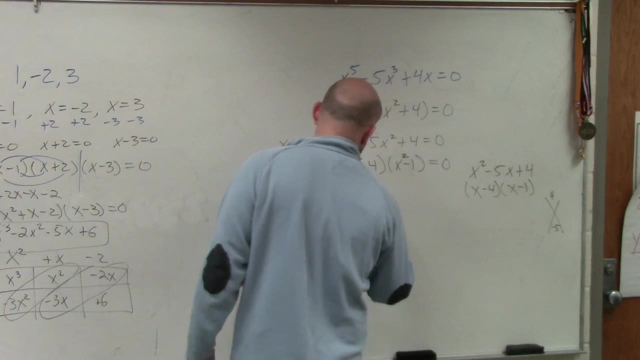 So x squared plus negative 1 times x squared gives you negative 5x squared. Now I can apply the zero product property again. So I'd say x squared minus 4 equals 0.. And x squared minus 1 equals 0.. 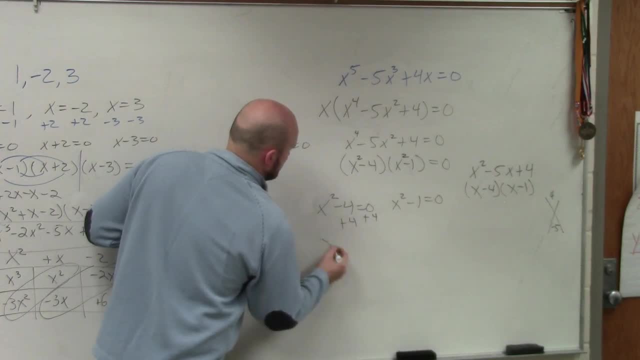 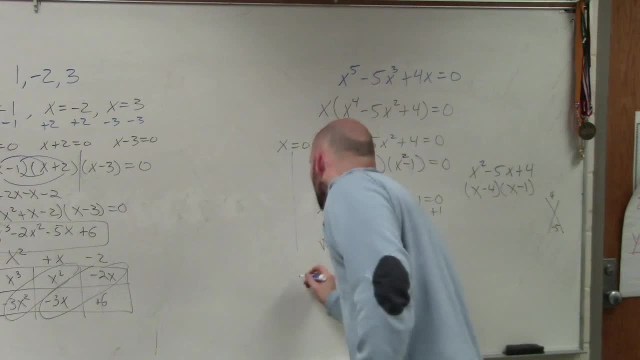 So my final answer is: x equals 0,, x equals plus or minus 2, and x equals plus or minus 1..